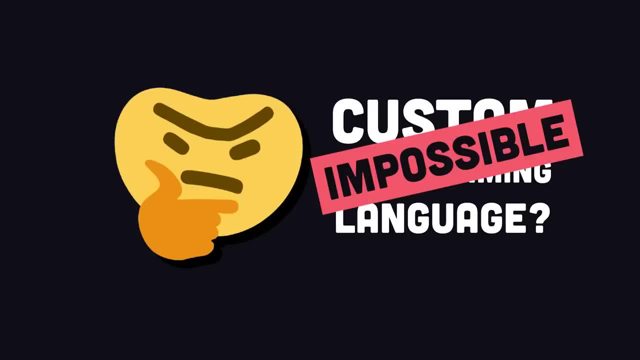 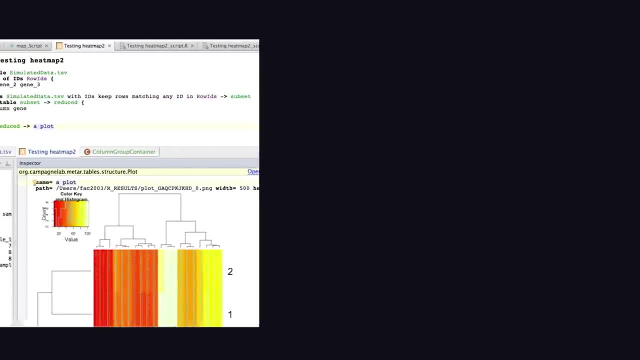 developer. building a custom-made software is a great way to build a software that can be used to build a custom programming language sounds like an impossible challenge. However, with this open-source IDE from JetBrains, anyone can build their own domain-specific language like MetaR, which is a highly specialized language for biomedical students who would. 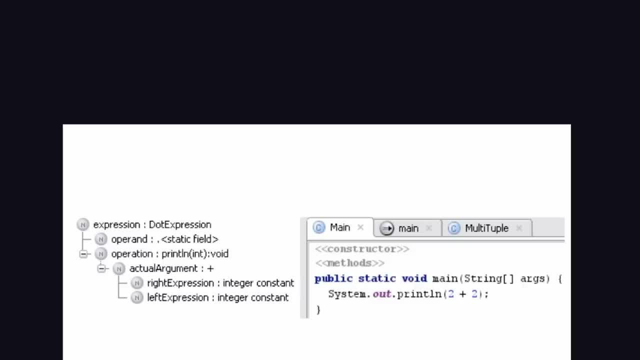 otherwise have to learn how to program in R JetBrains. MPS is a logical editor as opposed to a text editor, allowing end-users to interact with the code visually. This allows non-programmers to easily integrate their own domain logic. Then MPS will generate the code for the underlying 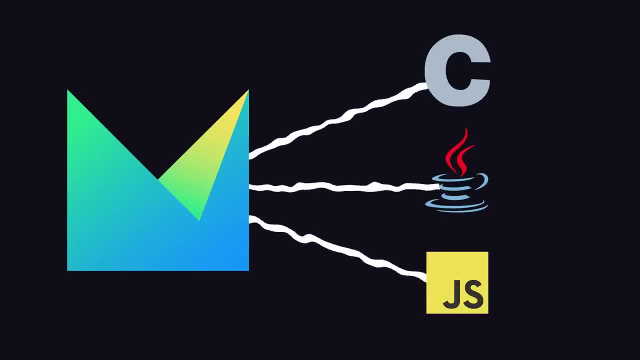 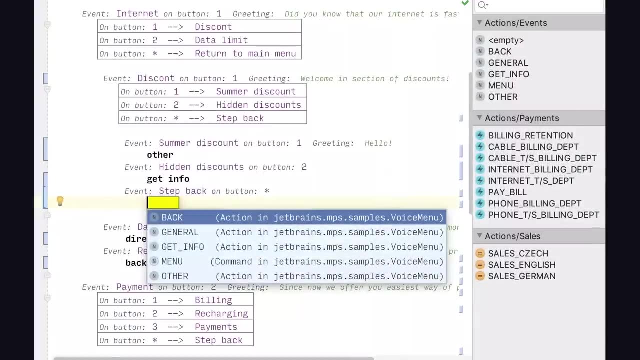 platform like C, JavaScript or any other language. That means anyone in the organization can harness the power of code in a safe, easy-to-learn environment, along with all the awesome tooling you would expect, like code completion, debuggers and more, To get started. 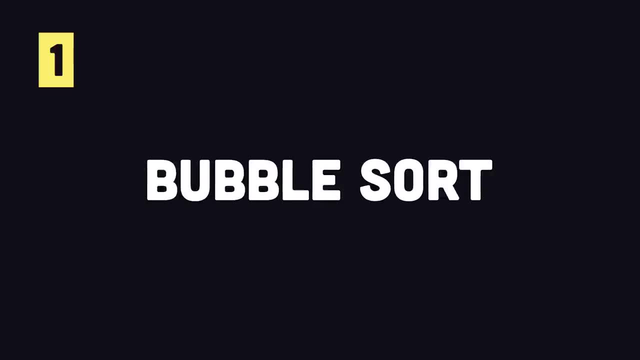 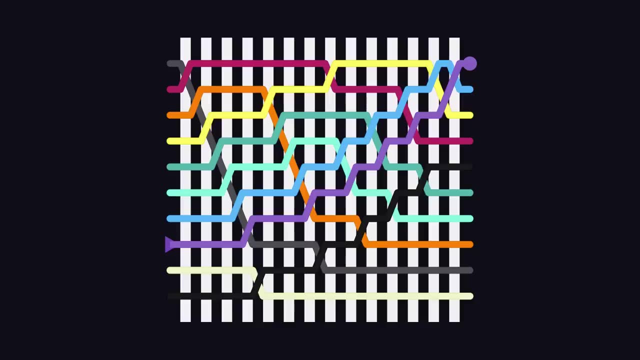 simply download it for free and give it a try. Now back to the program. The first algorithm we'll implement is BubbleSort, which, in my opinion, is the easiest one to wrap your head around. It works by comparing adjacent elements, then swaps them if they're in the wrong order, which allows smaller. 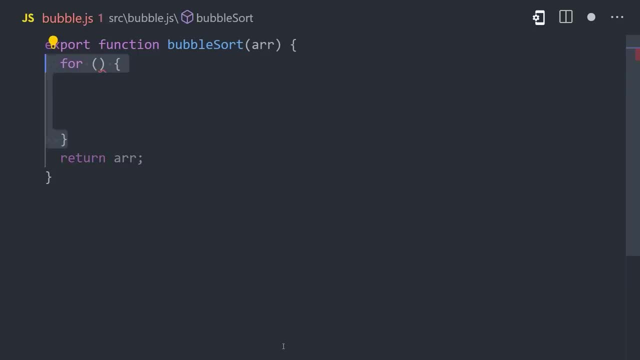 elements to bubble to the top of the list. First we'll set up a for loop for the length of the array, inside of which we'll nest another loop that loops over the array minus the current loop. In this loop we can do swapping by comparing the current index to the one next to it, If the left 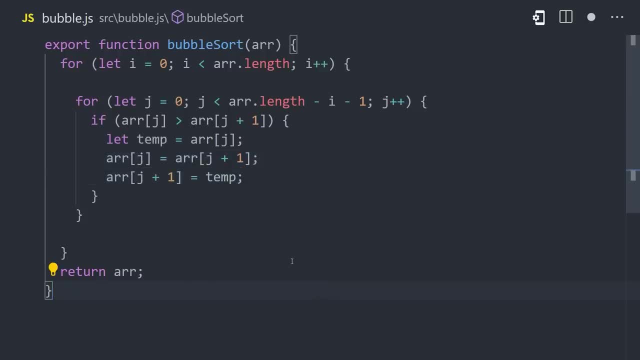 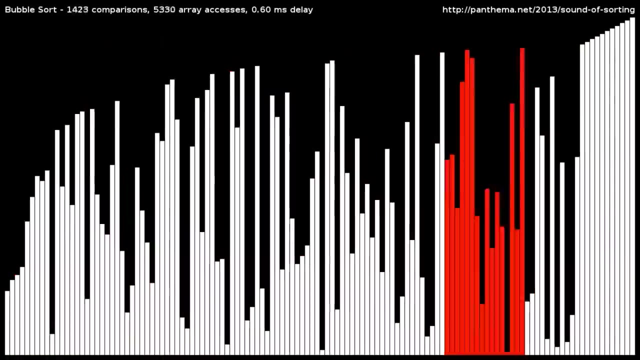 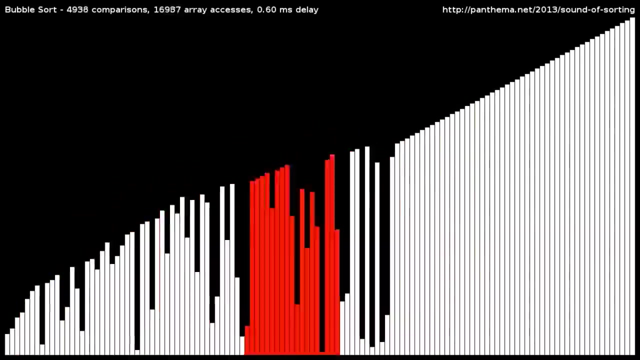 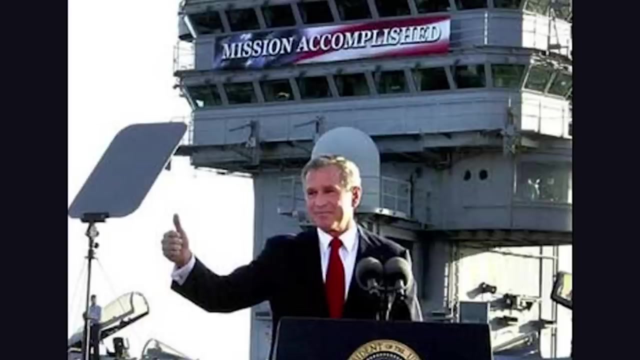 side is greater than the right side, then they'll need to trade places. The process continues until we go through the entire outer loop. And here's what it looks like: BubbleSortcom. BubbleSort is intuitive but not very performant. Its average time complexity is O of n squared. 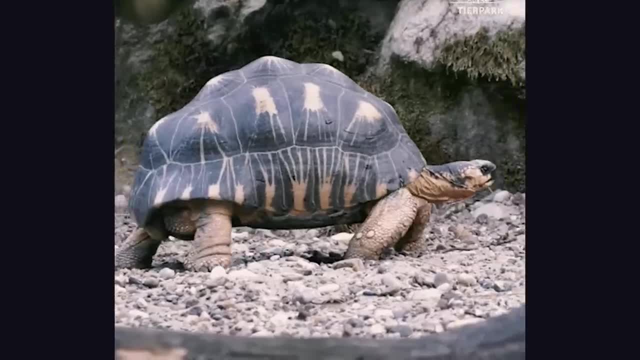 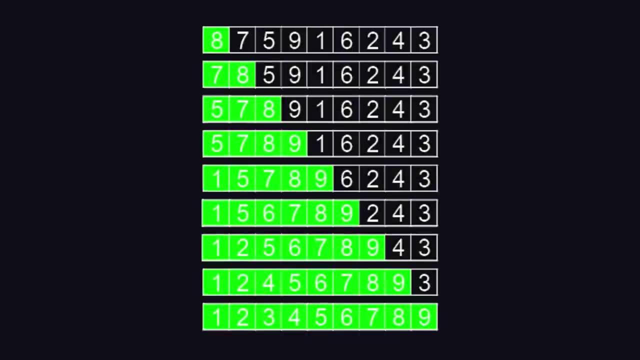 or quadratic time, which gets slower and slower as the list grows longer. This won't cut it in the real world. Another fairly easy option to implement is InsertionSort, which builds up a sorted array one element at a time. Once again, we start with a loop, but this time we start at. 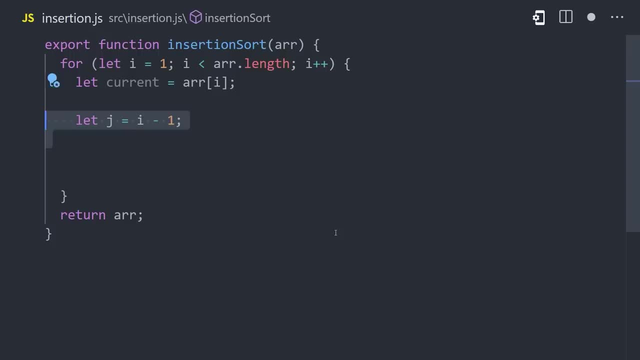 index 1, or the second value in the array. We then set up variables for the current value and previous index, and while the previous index is greater than the current value, we move the previous value to the right, Then we move to the left until we find a previous value, and then we 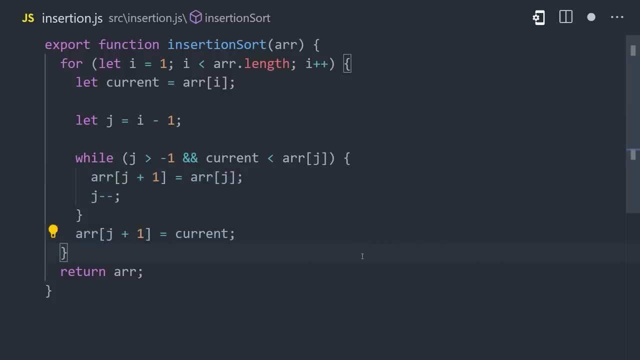 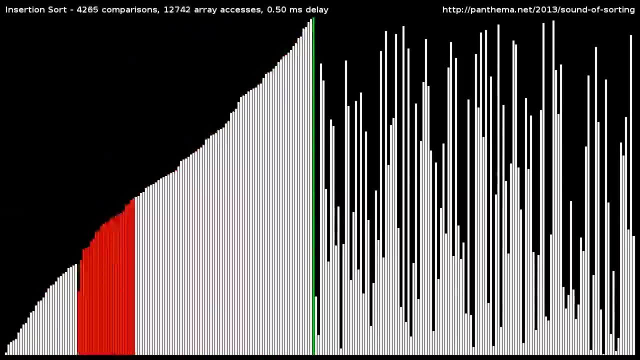 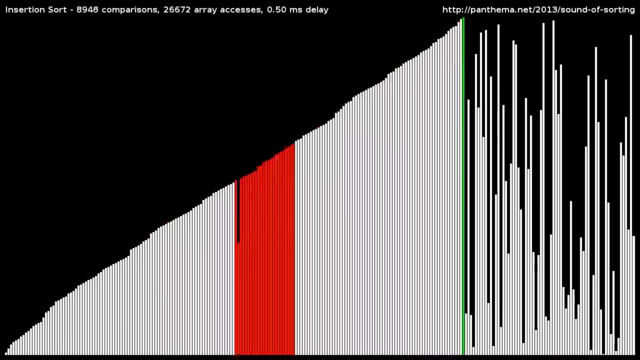 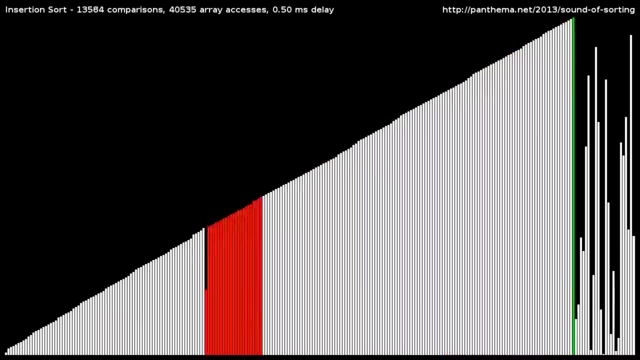 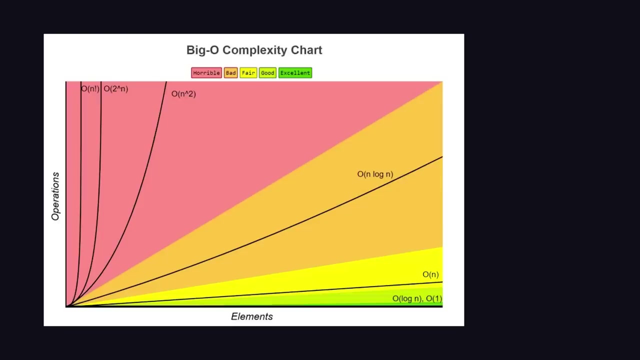 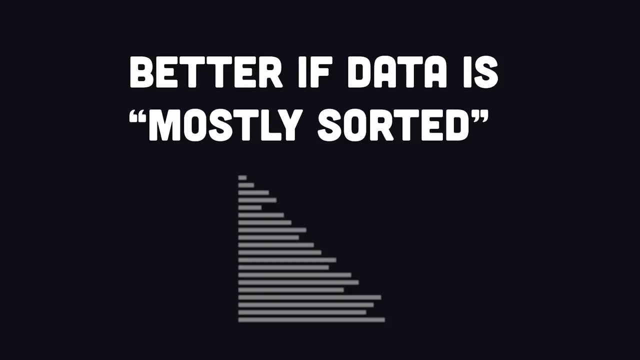 value that is smaller, at which point we can insert the current element. Here's what it looks like in action. Once again, we have a nested loop here, which results in quadratic time complexity, but in practice it can still be pretty fast if the input data is already mostly sorted. 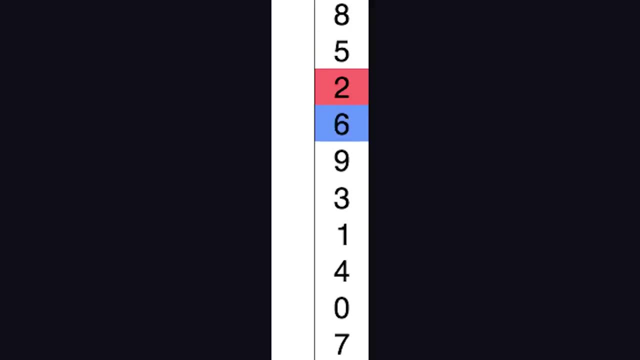 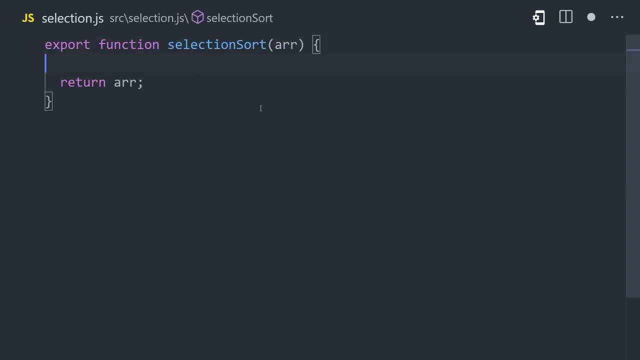 Another similar approach is SelectionSort. It works by finding the smallest element in the array and exchanges it with the element at the beginning, then repeats this process until it's fully sorted. Once again, we loop over the entire array and then add a nested loop inside of it. 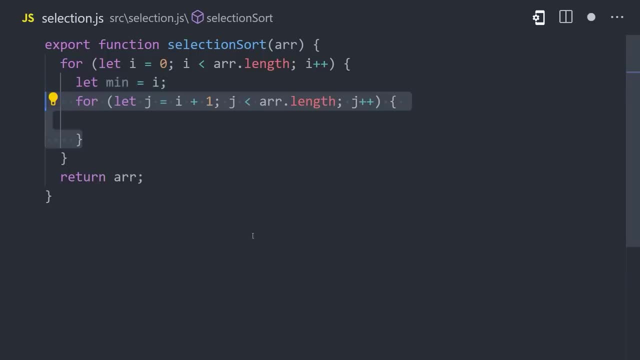 but this time we're looking for the minimum value in the subarray in this nested loop. If the minimum value doesn't equal the current value, then we swap them out, which will effectively put the smallest element in the proper position, then repeat that process across the entire array. Let's check it out. 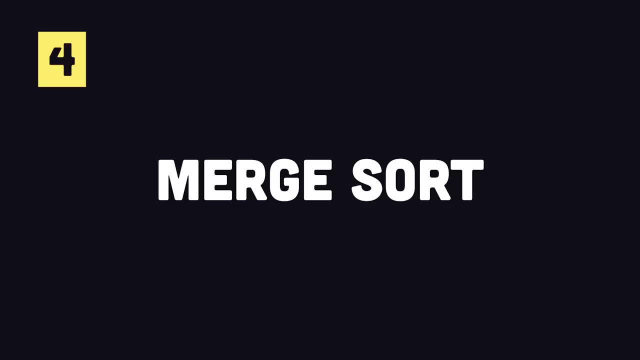 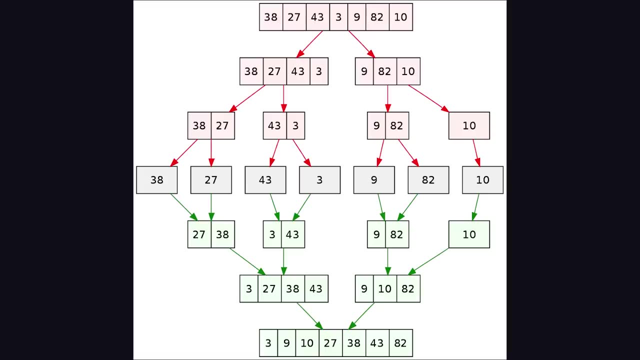 And MergeSort also results in quadratic time. Next up we have MergeSort, which is a divide and conquer algorithm that's been around since the 1940s. The idea is to break the main array into subarrays, sort them and then merge them back together. Unlike the other examples we've 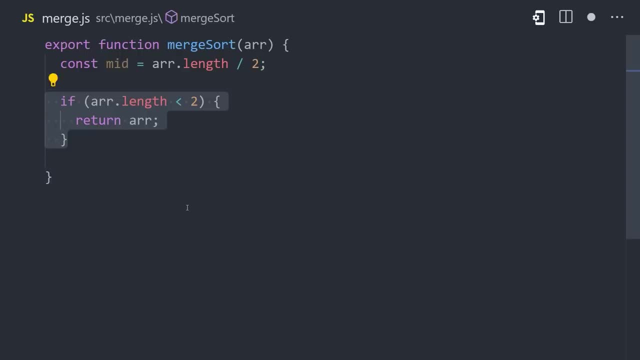 looked at this. one is implemented recursively. First the recursive function finds the midpoint of the array. then we have a base case here that will stop the loop when the array length is less than 2. We then break the array in half at the. 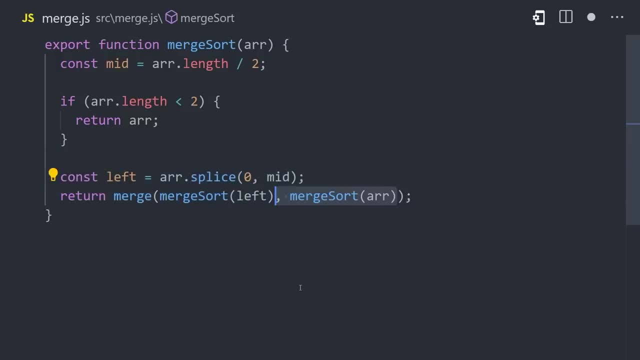 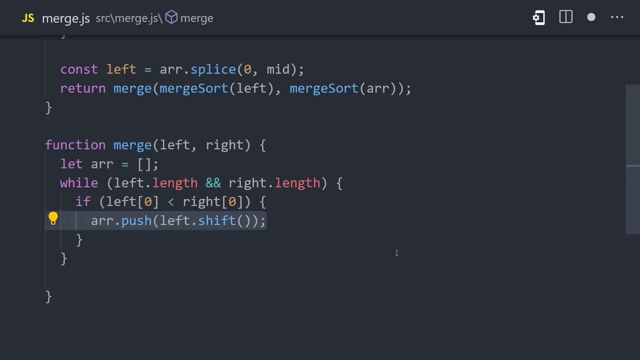 midpoint using splice, and then we call the same function on both halves. But in order for that to work, we'll also need to implement a merge function that does the actual sorting. It loops over both arrays simultaneously, compares their values and adds them in order to a new array. Then finally, 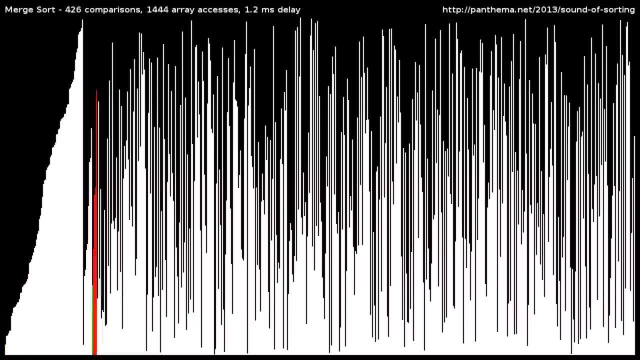 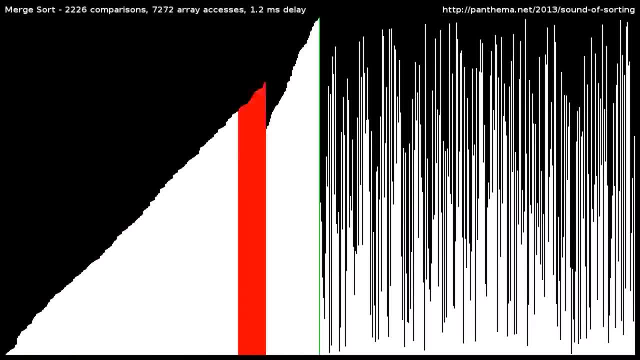 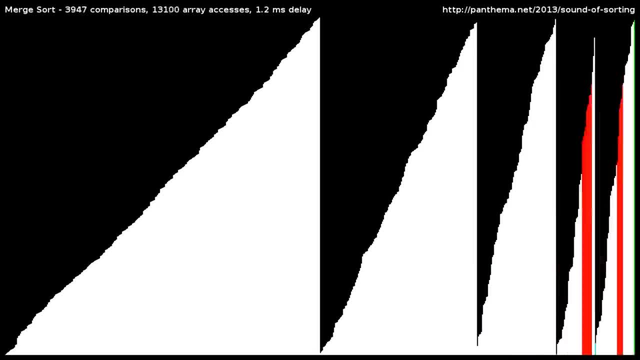 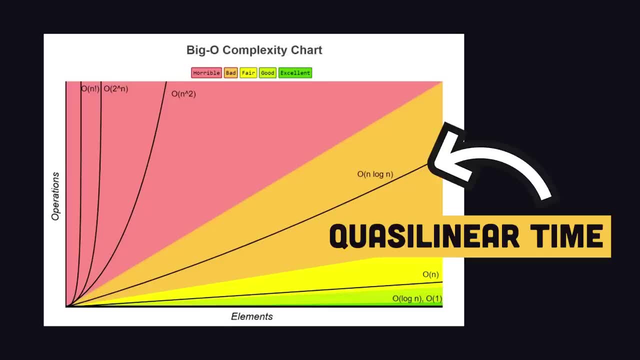 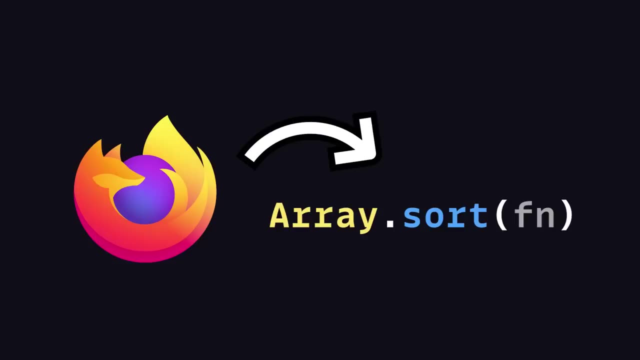 it merges everything back together. Here's how it looks. It's a bit more complex to implement but performs much better at quasi-linear time. That's why a variation of MergeSort is the algorithm implemented under the hood for array sort in JavaScript. 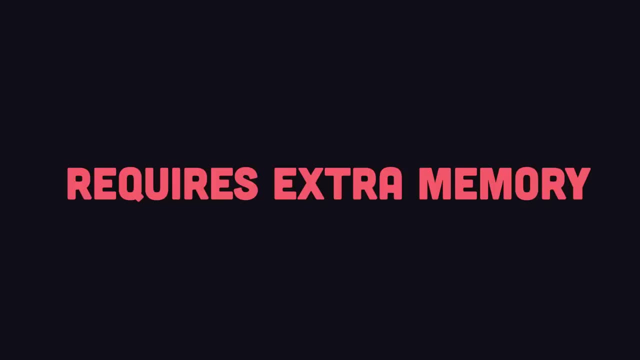 as well as many other languages and applications. One drawback, though, is that it doesn't sort in place and requires a lot of time to do so. So if we're going to do a merge sort, we're going to have to split the array in half. If that's a problem, a similar alternative option is Quicksort. 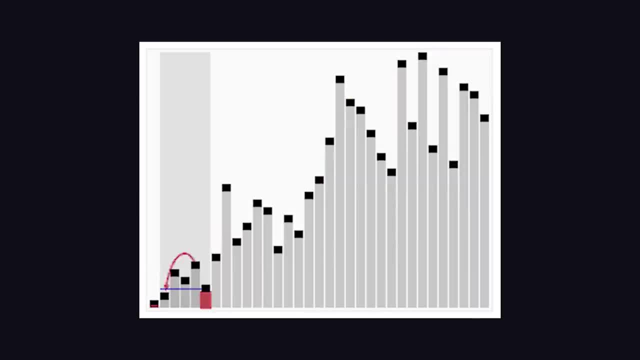 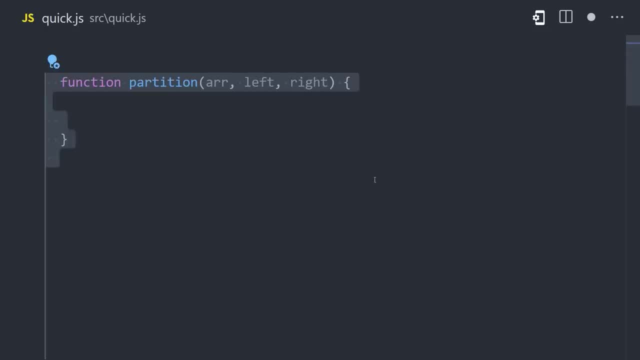 It's also a divide-and-conquer algorithm that uses a pivot element to create subarrays that are sorted recursively. With Quicksort, the array isn't necessarily split in half and works with any ratio. To sort the array in place, we'll first create a function called 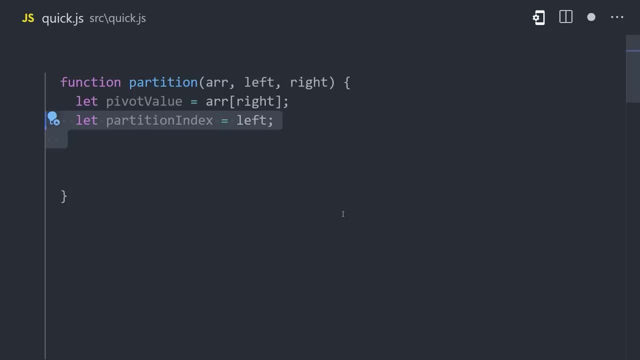 partition. Its job is to divide the array into two parts, to separate the element smaller than the pivot from the values greater than the pivot. In this case, the pivot value is set to the element at the right index of the array. From there we loop over the portion of the array between the 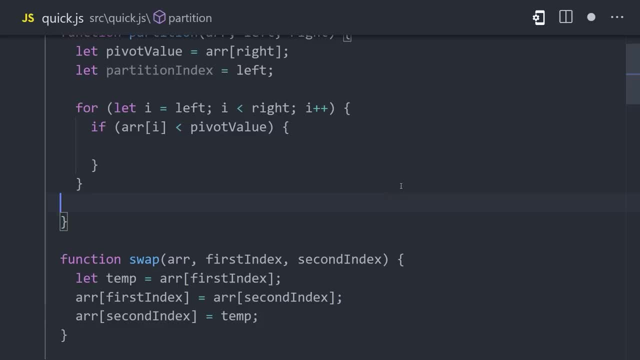 left and the right. If we want to sort the array in place, we'll first create a function called partition. If we want to sort the array in place, we'll first create a function called left-and-right values. If a value is less than the pivot value, then we swap it with the element. 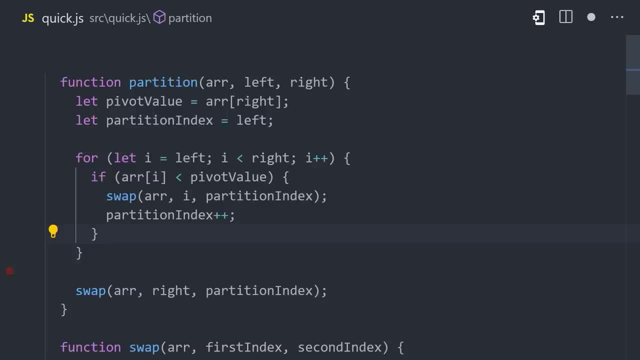 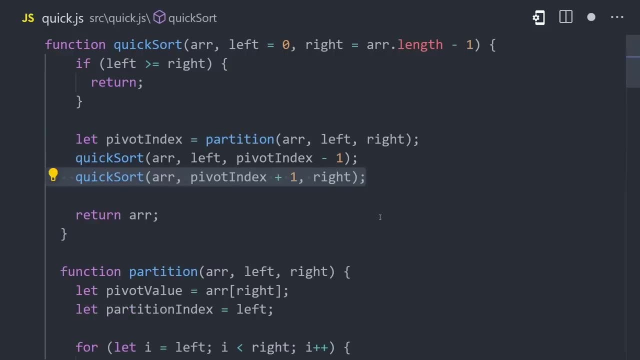 at the partition index. From there we can create a recursive function called Quicksort to divide and conquer both the left and right side of the array. This is the more proper way to implement Quicksort, but we can illustrate the concept a little better by cheating In this more simplified 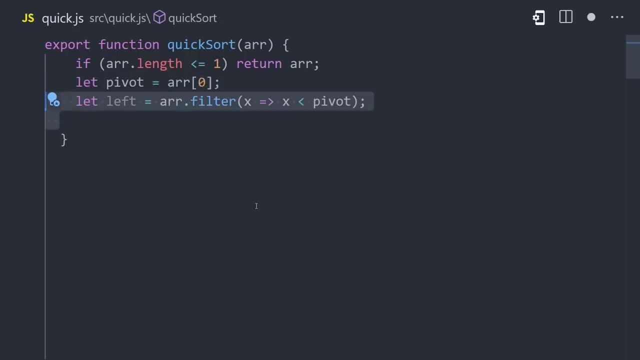 function. notice how I'm first determining a pivot point on the array. then we divide and conquer by filtering out items that are less than the pivot on the left side and items that are more than the pivot on the right side. Now call that recursively to sort the entire array. That 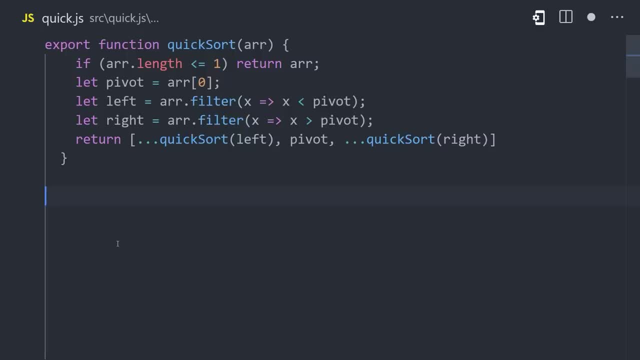 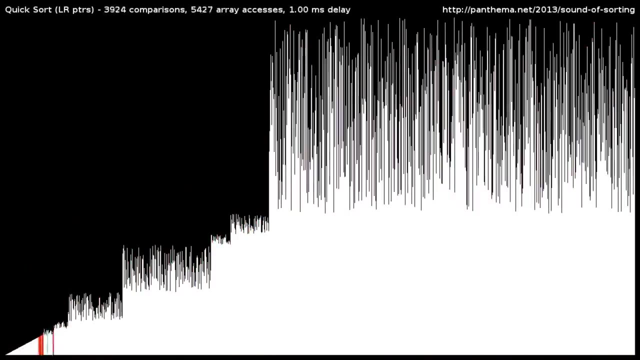 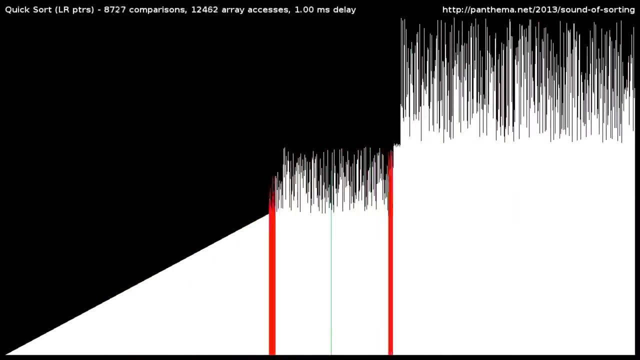 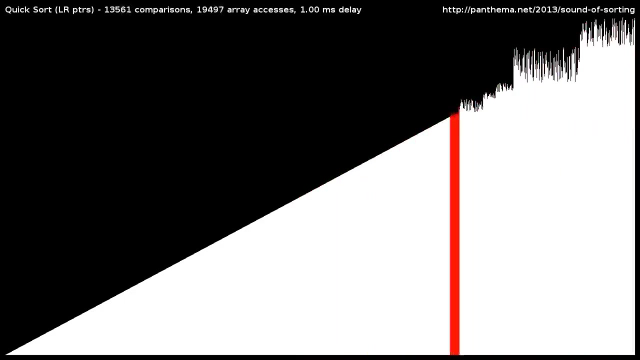 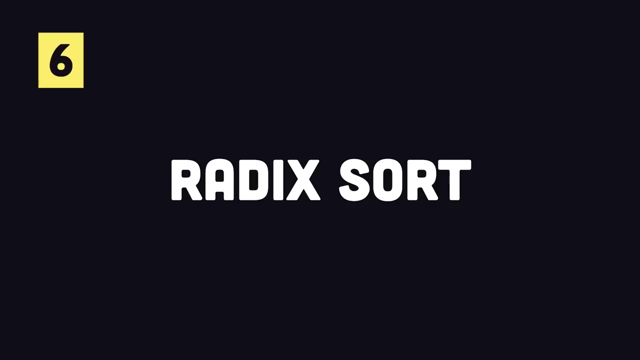 works, but it won't perform as well as the previous implementation. In any case, let's go ahead and watch it on TV. Next up we have RadixSort, which was created all the way back in the 1800s for tabulating. 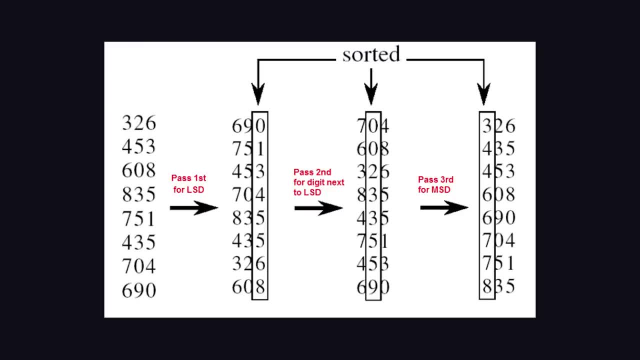 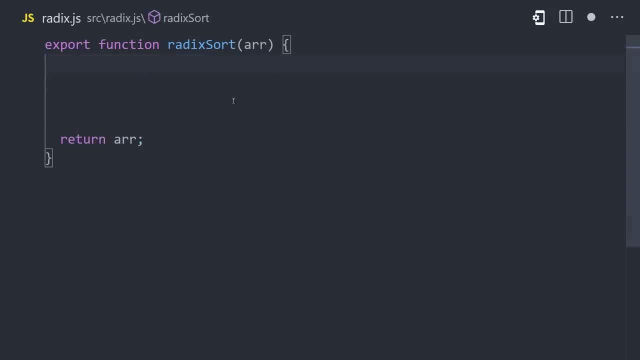 machines. It's still used today on values like integers or binary strings, because it takes a unique approach where it groups items that share the same significant position or place value. The implementation's a bit more complex, but basically it works like this: It splits the. 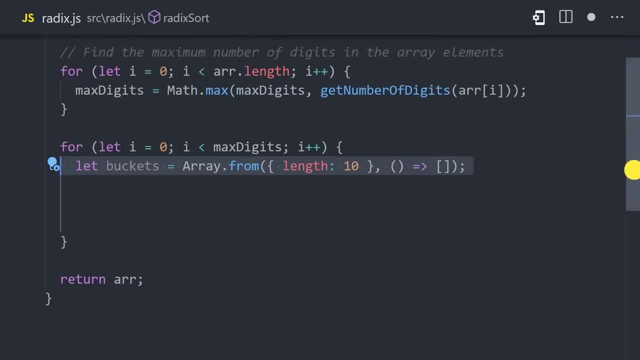 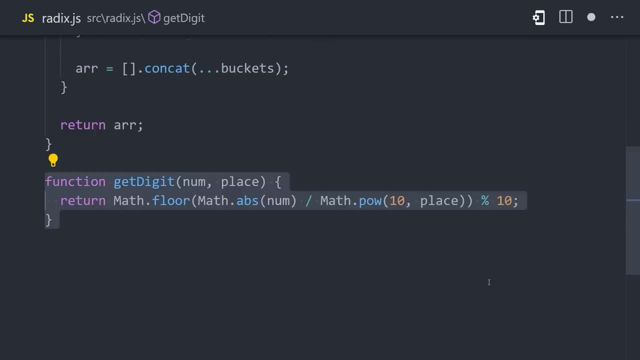 elements of the array into 10 buckets, one for each digit, 0 through 9.. It then loops over those buckets and has a nested loop for the array itself. GetDigit will then find the number at that place, going from 0 to 9, which provides a nested loop for the array itself, GetDigit. 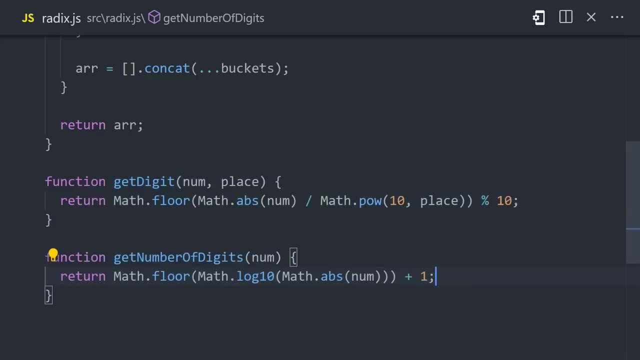 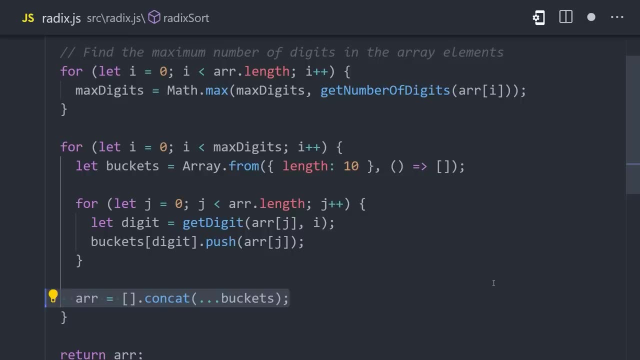 has a bunch of sorted buckets that are combined back into the original array. What's interesting here is that there's no direct comparison going on. We're only looking at the underlying digits. This implementation is called LSD, or least significant digit, but it's also possible to